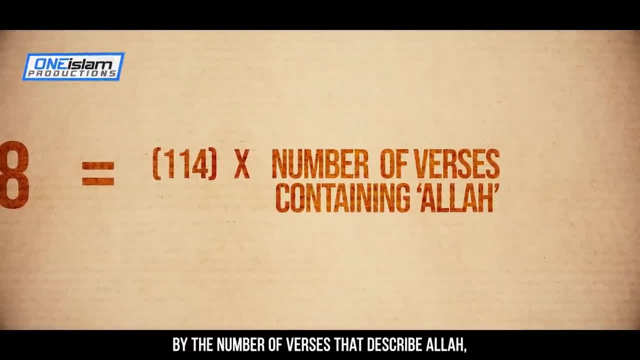 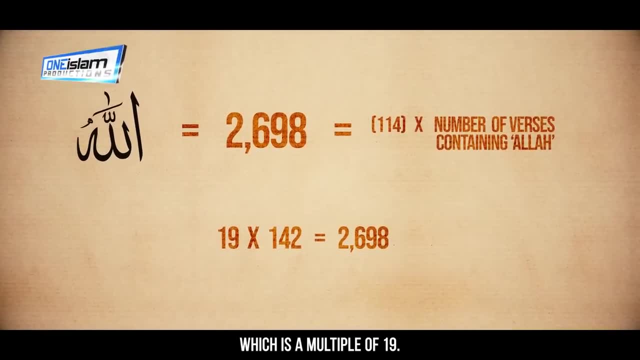 by the number of surahs in the Qur'an, the number of surahs in the Qur'an will be 2,698 times. If we multiply by the number of verses that describe Allah, we get 2,698. Which is a multiple of 19.. 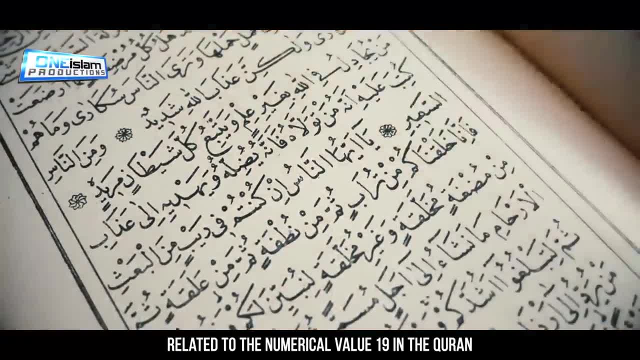 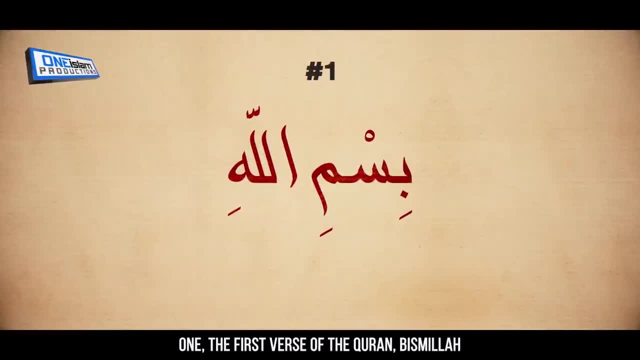 There are several intriguing facts related to the numerical value 19 in the Qur'an. 1. The first verse of the Qur'an, Basmala, consists of 19 letters. 2. The Qur'an includes one verse of the Qur'an, which is membership. Bは إله, b Dan ق sigh sin c Nororish I Parker Tsk Bukha Bur'u kes m. Musicftein福aa Tein bergahou, Taq quá Sittaranaafternafalih scores Вамi »ẓamunби. 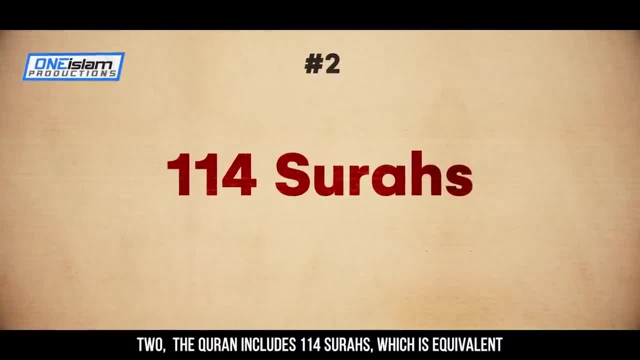 Swing by the number of verses that describe Allah. we get 2698, which is a multiple of 19.. There is several intriguing facts related to the numerical value. 19 in the Qur'an includes 114 surahs, which is equivalent to 19 multiplied by 6.. 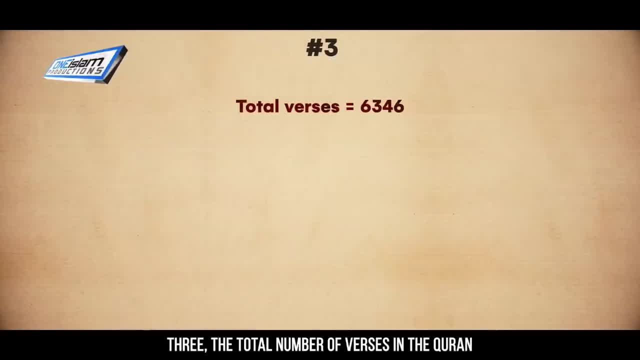 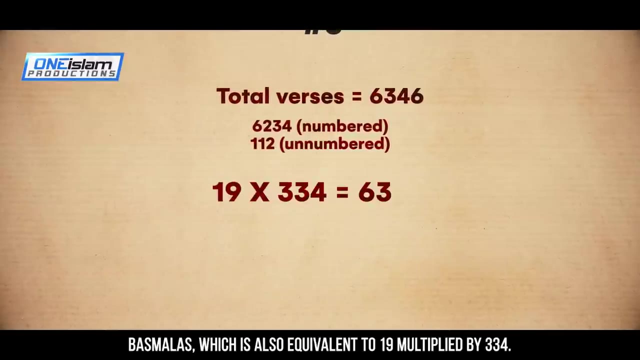 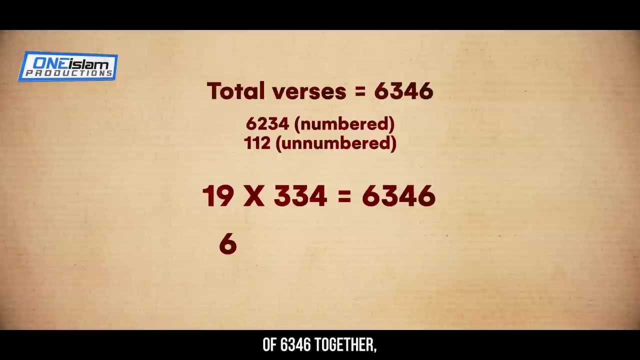 3.. The total number of verses in the Qur'an is 6346, with 6234 numbered verses and 112 unnumbered verses, which is also equivalent to 19 multiplied by 334.. It is interesting to note that when we add the digits of 6346 together, 6 plus 3 plus. 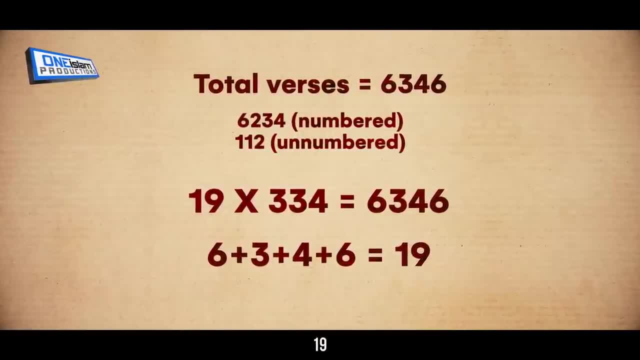 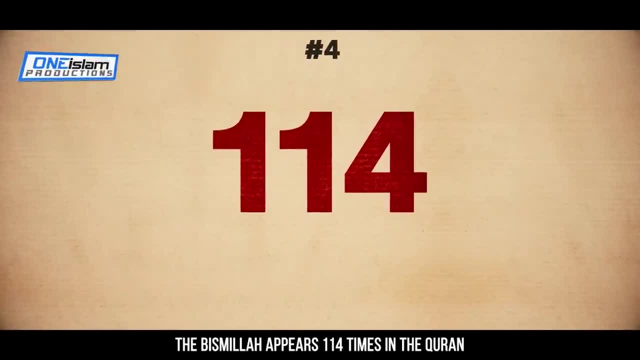 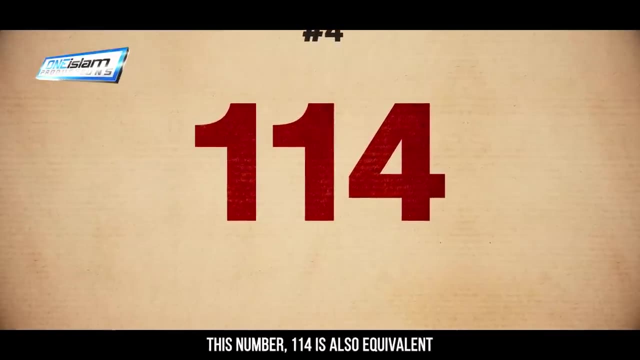 4 plus 6, we get the value 19.. 4.. The basmala appears 114 times in the Qur'an, except in surah 9, where it is missing but occurs twice in surah 27.. This number 114 is also the number 114 in the Qur'an. 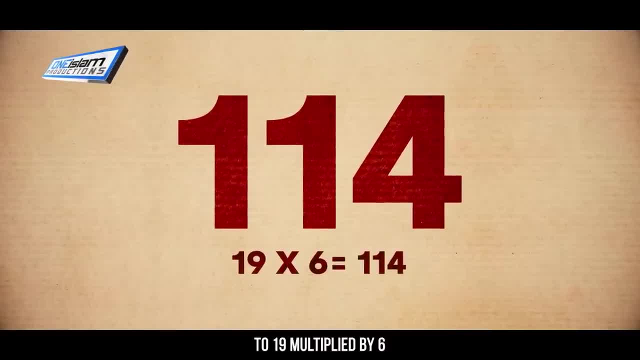 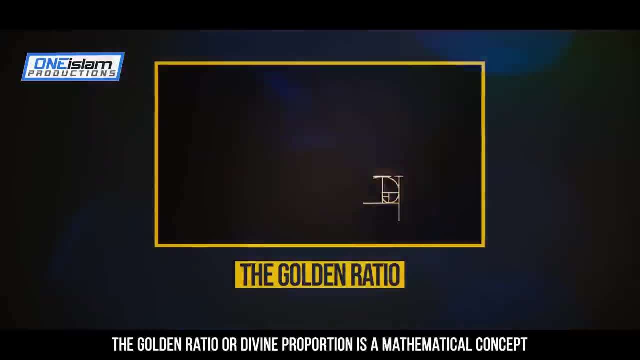 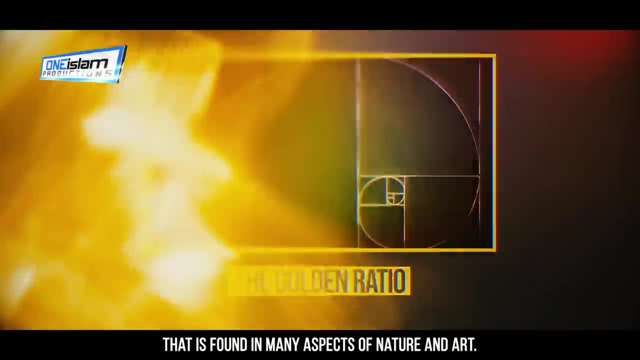 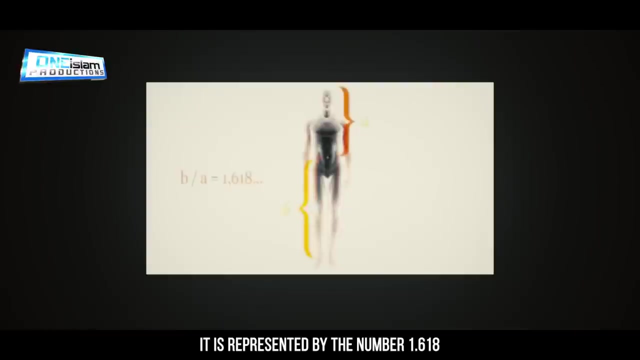 It is also equivalent to 19 multiplied by 6. 2. The Golden Ratio, The golden ratio, or divine proportion, is a mathematical concept that is found in many aspects of nature and art. It is represented by the number 1.618 and can be seen in the proportions of the human. 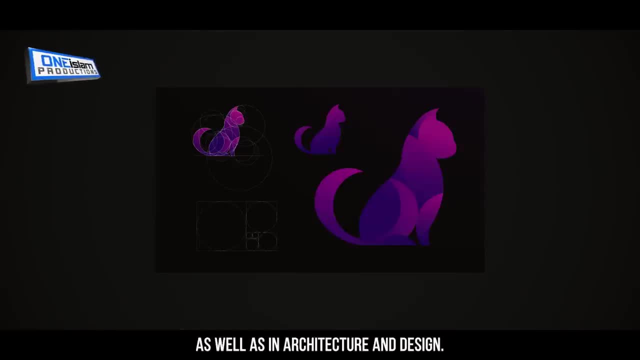 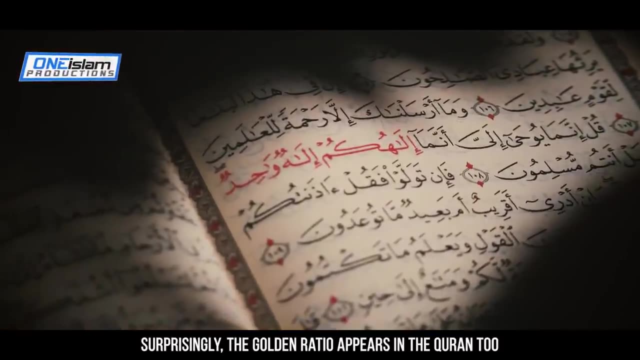 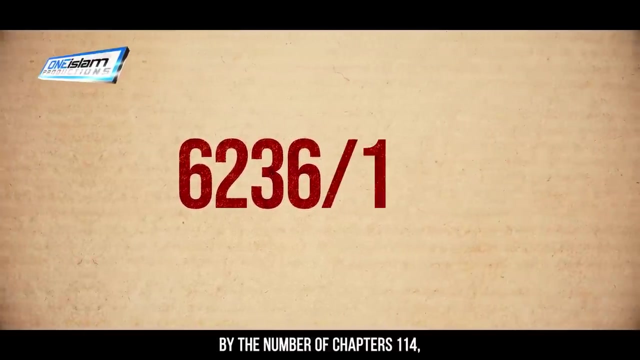 body. The golden ratio is the number of verses in the Qur'an, as well as in architecture and design. Surprisingly, the golden ratio appears in the Qur'an too. If we divide the number of verses in the Qur'an- 6236,- by the number of chapters- 114,- we get. 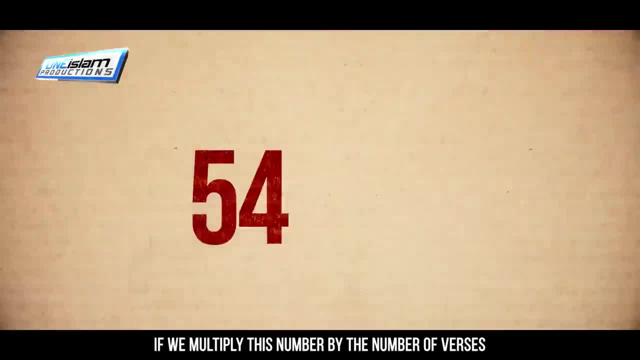 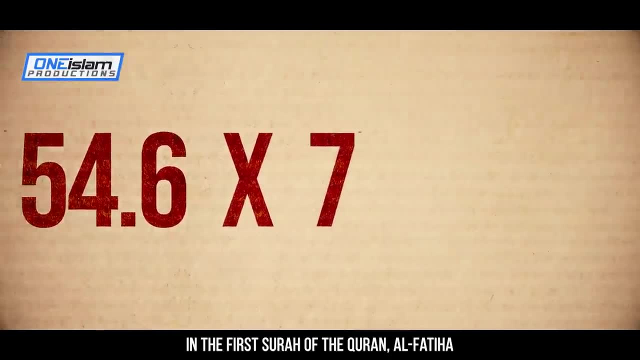 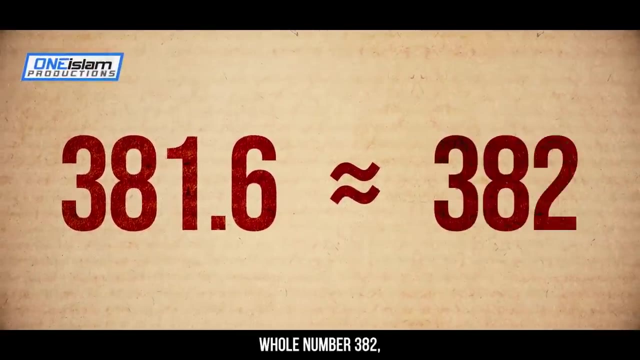 54.6.. If we multiply this number by the number of verses in the first surah of the Qur'an Al-Fatiha, we get 54.6.. We get 381.6.. If we round this number to the nearest whole number, 382, we get a remarkable result. 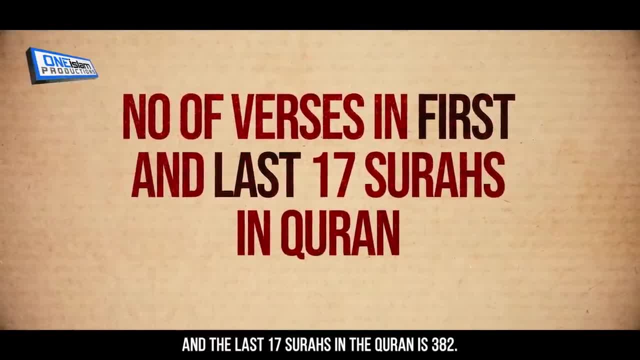 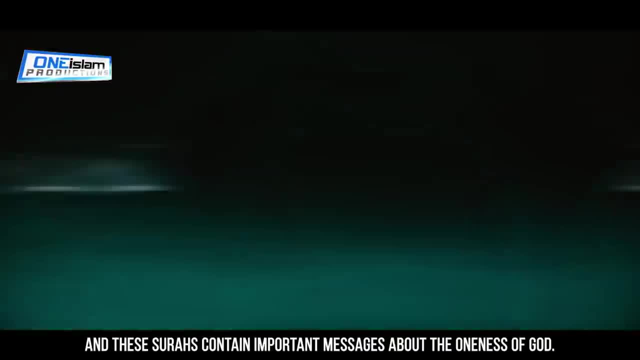 The total number of verses in the first and the last 17 surahs in the Qur'an is 382.. And these surahs contain important messages about the oneness of God, the Day of Judgment and other topics. The Qur'an is 382.. 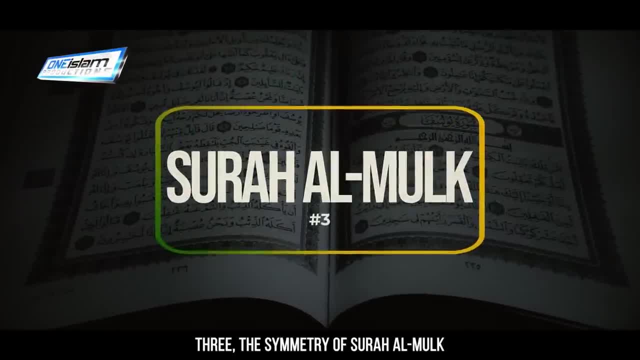 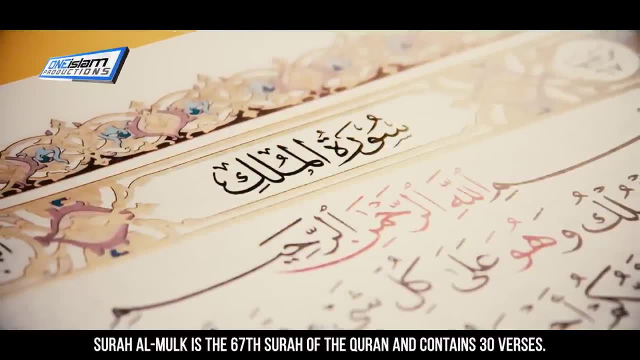 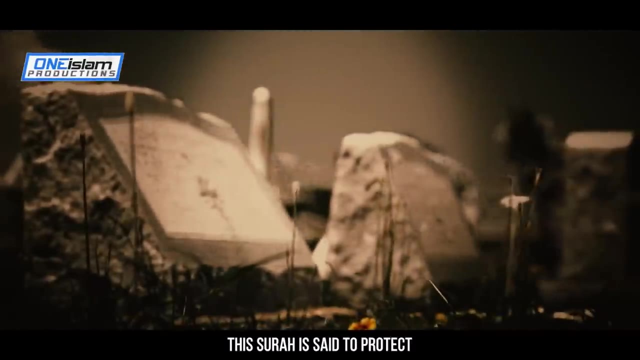 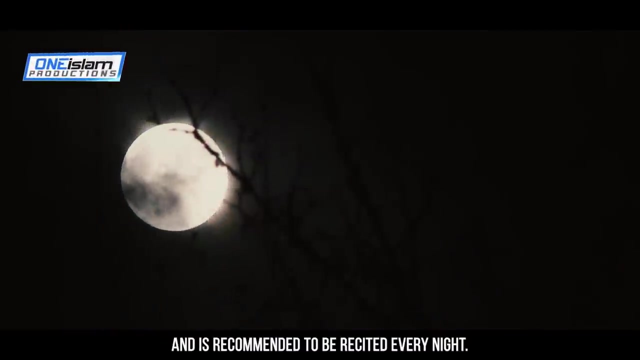 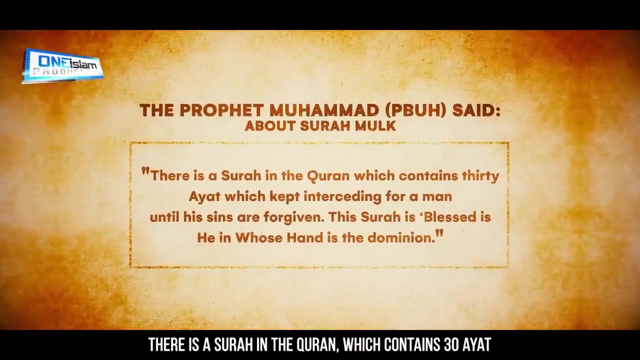 It says Thebase 49.. The surah is said to protect its reciter from the punishment of the grave and is recommended to be recited every night. The Prophet Muhammad said a surah in the Quran which contains 30 ayat, which kept interceding for a man until his. 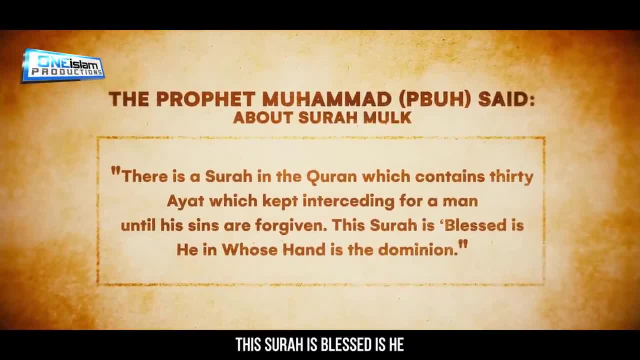 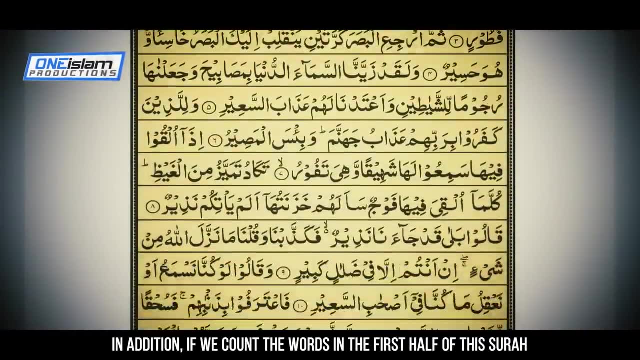 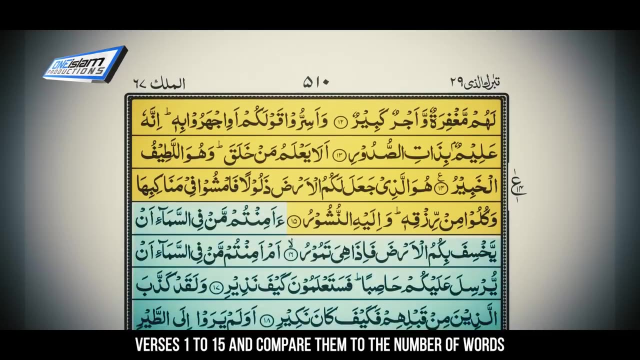 sins are forgiven. This surah is: blessed is he in whose hand is the dominion. In addition, if we count the words in the first half of this surah- verses 1-15, and compare them to the number of words in the second half- verses 16-30,, we find that they are equal. 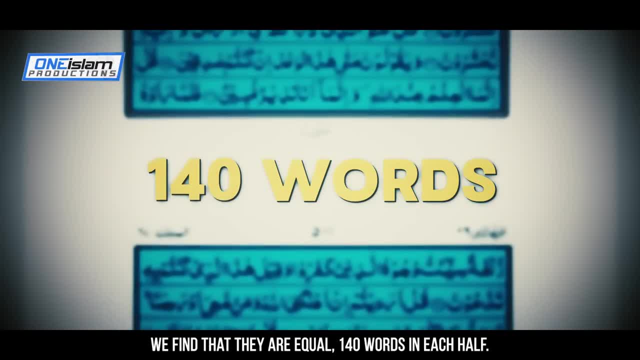 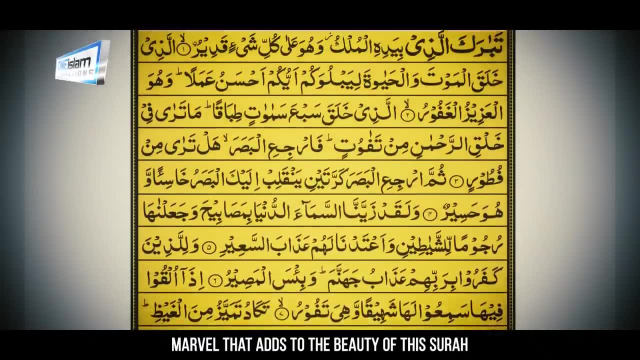 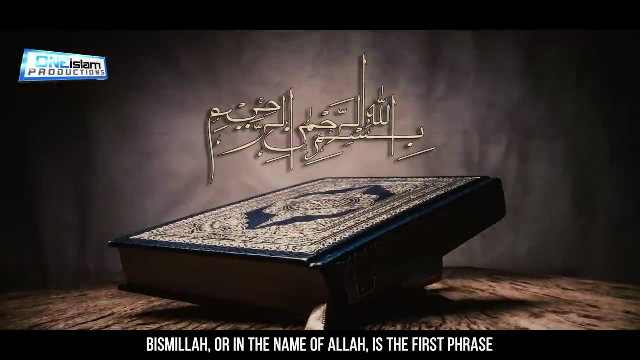 140 words in each half. The symmetry is a mathematical marvel that adds to the beauty of this surah, 4.. Numeric Value of Bismillah. Bismillah, or in the name of Allah, is the first phrase in every surah. 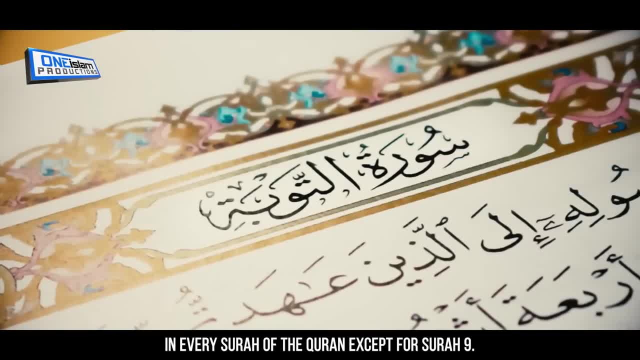 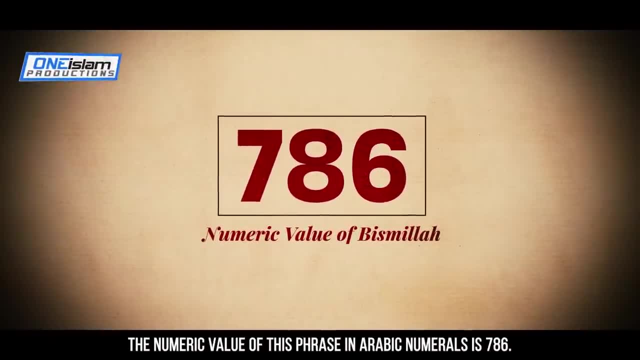 Bismillah, or in the name of Allah, is the first phrase in every surah. Bismillah, or in the name of Allah, is the first phrase in every surah. The numeric value of this phrase in Arabic numerals is 786.. The number has been revered. 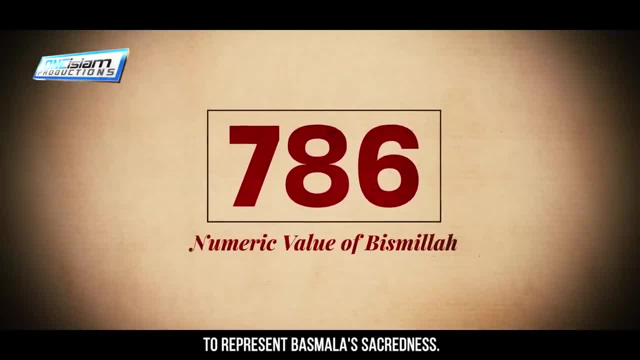 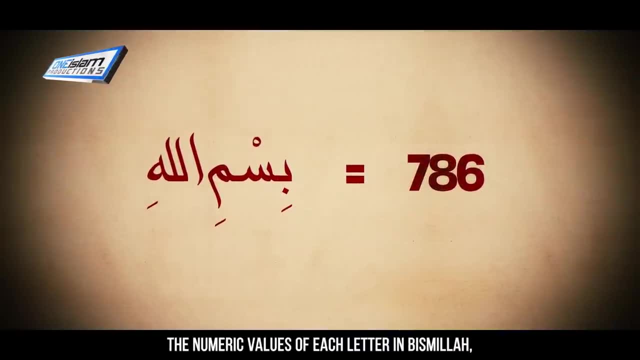 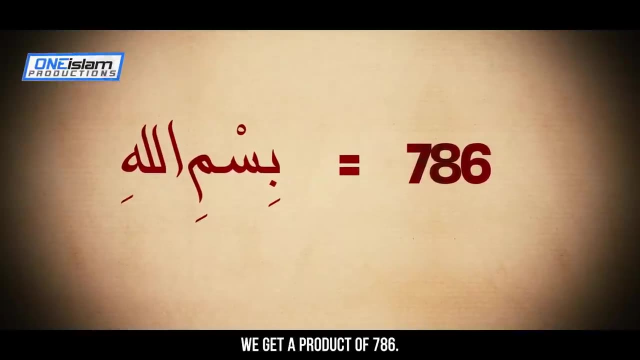 by many Muslims and is considered to represent Basmala's sacredness. Interestingly, if we multiply the numeric values of each letter in Bismillah, we get a product of 786.. This phenomenon has encouraged Muslims to recite this phrase regularly, as they believe. 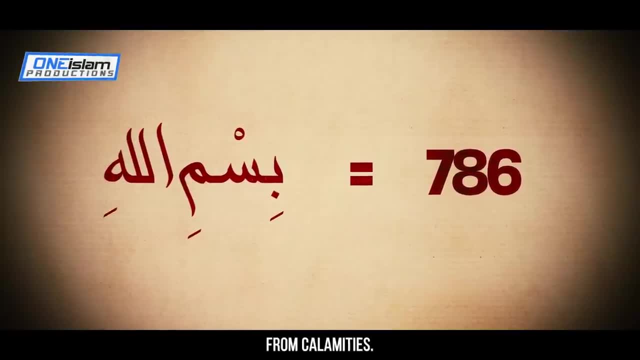 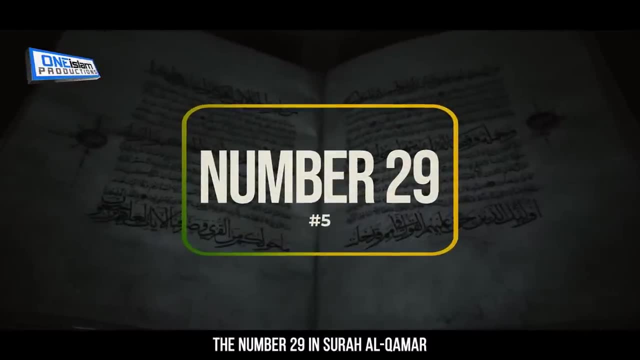 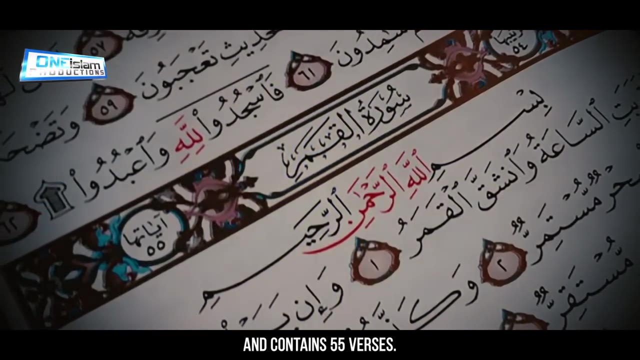 that it brings blessings and protection from calamities. 5. The number 29 in Surah Al Qamar. Surah Al Qamar is the 54th surah of the Quran and contains 55 verses. This surah describes the punishment that before the Qur'an was given to the Muslims. The surah is the punishment. 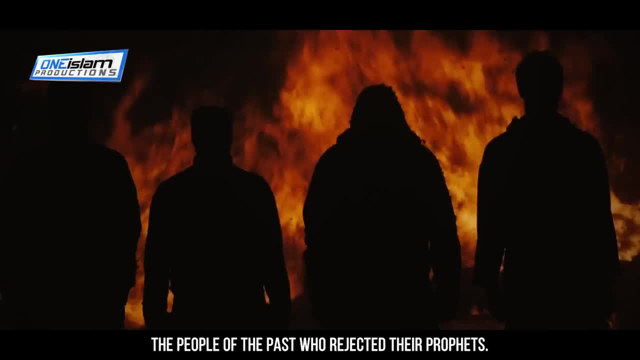 that before the Qur'an was given to the Muslims. The surah is the punishment that before the Qur'an was given to the Muslims. This surah is the punishment that before the Qur'an was given to the Muslims. The surah is the punishment that before the Qur'an was given to the Muslims. 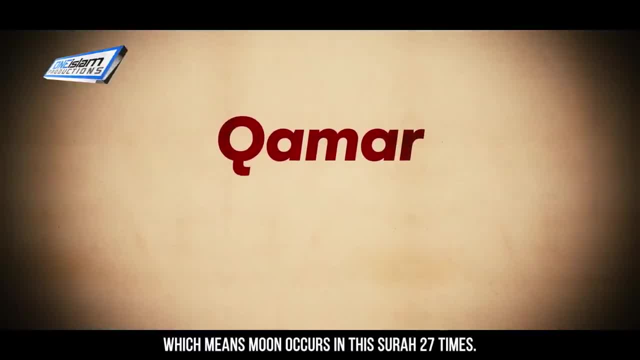 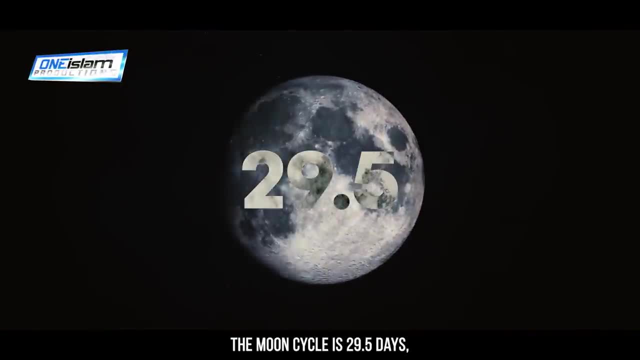 Interestingly, the word Qamar, which means Moon, occurs in this surah 27 times. Very interestingly, the verd plead: きمَرAND личتكر 죽ماً. The moon's cycle is 29.5 days. The number 29 is the ordinal value of the Qur'anic. 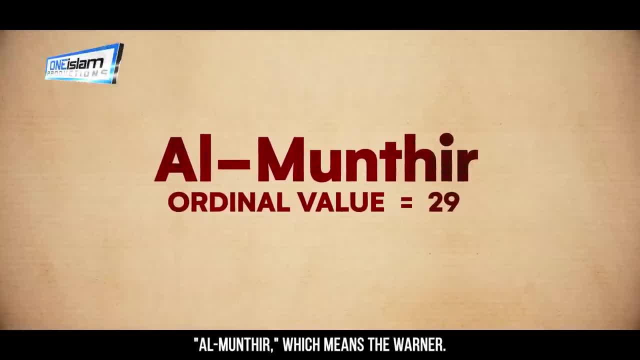 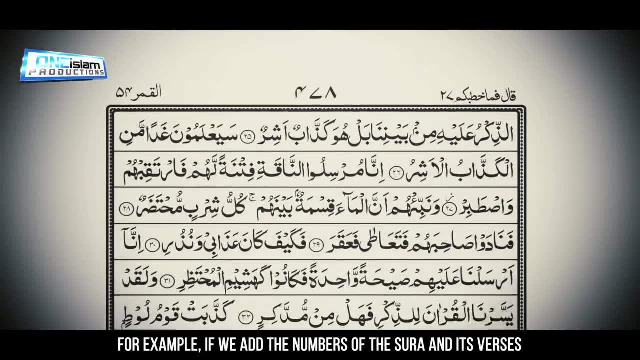 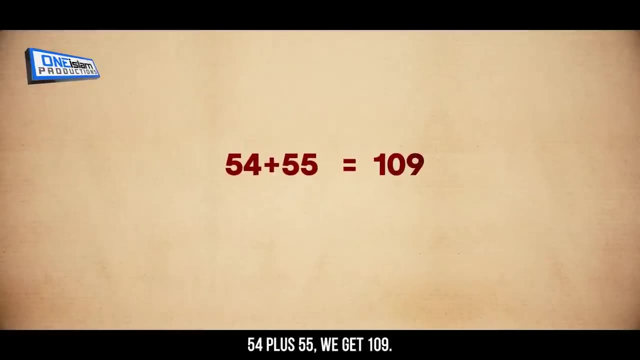 word 다니ل, the surah. for example, if we add the numbers of the surah and its verses, 54 plus 55, we get 109. if we subtract this number from the total number of chapters in the quran- 114, we get 5.. 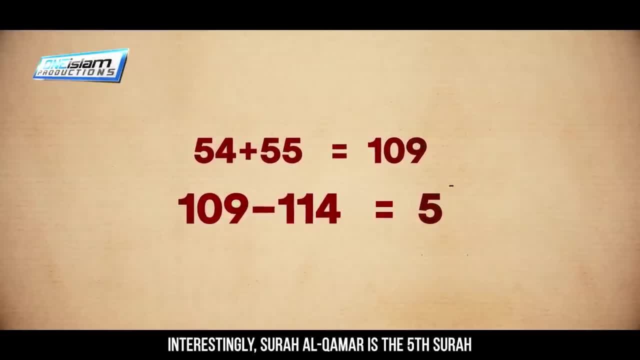 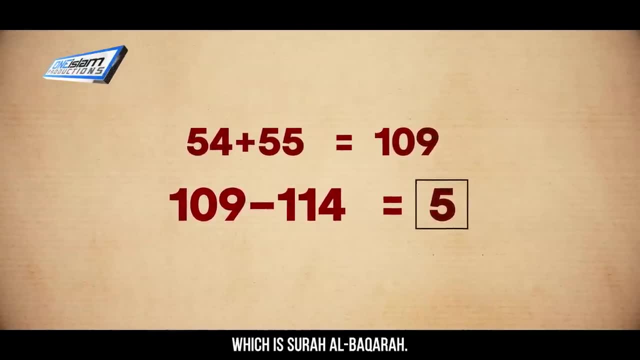 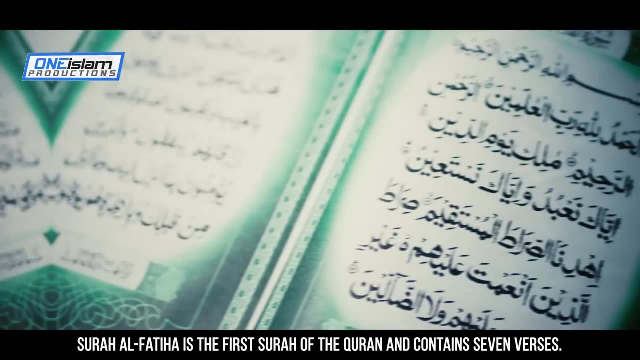 interestingly, surah al-qamar is the fifth surah after the last muqata'at surah of the quran, which is surah al-baqarah six, the number eight, in surah al-fatihah. surah al-fatihah is the first surah of the quran. 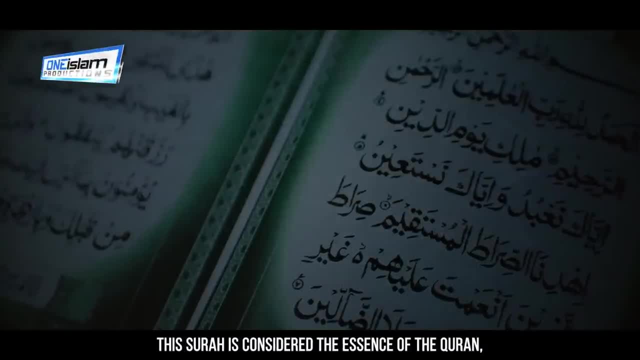 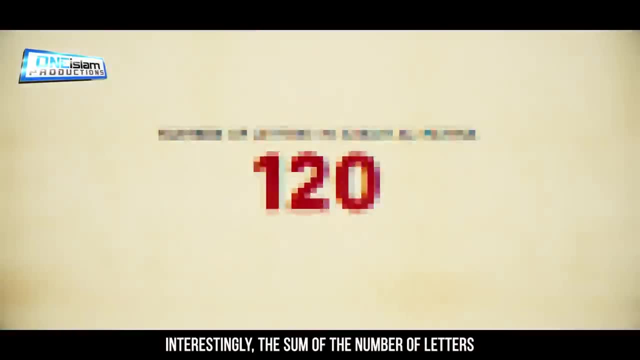 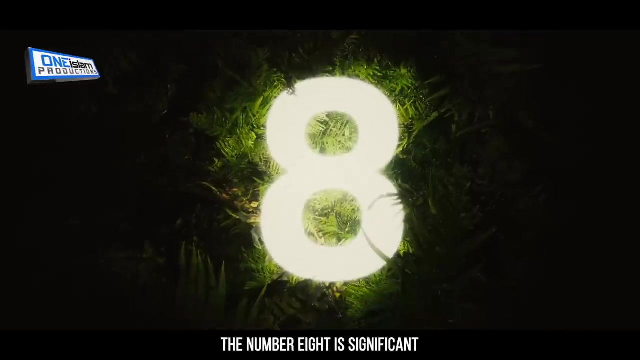 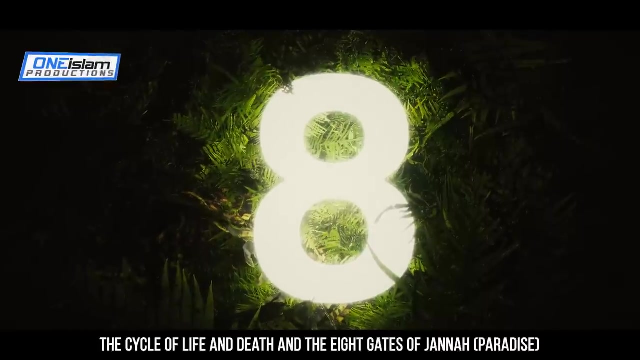 and contains seven verses. this surah is considered the essence of the quran and is recited in every prayer by muslims. interestingly, the sum of the number of letters in the surah is 120, which is a multiple of eight. the number eight is significant because it represents infinity, the cycle of life and death. 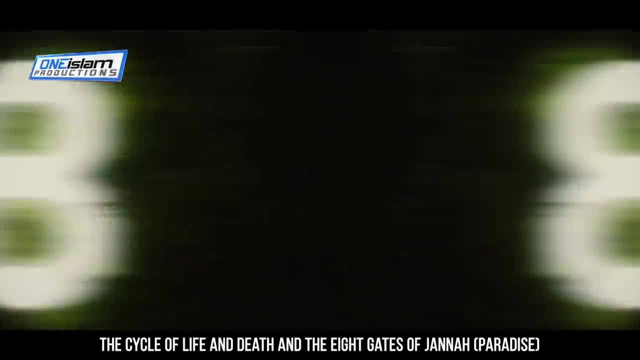 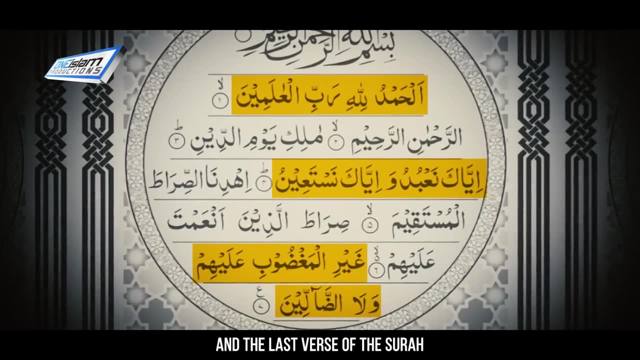 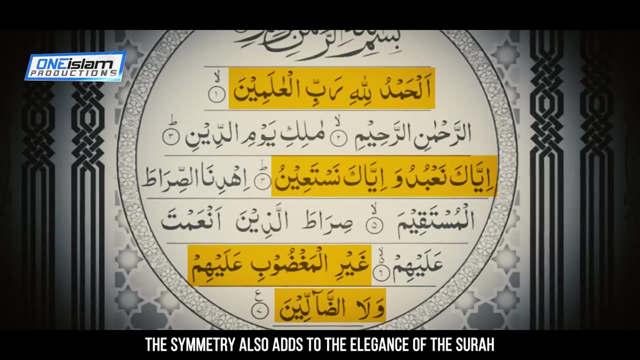 and the eight gates of jannah paradise. furthermore, if we count the number of letters in the first, middle and the last verse of the surah, we find that they are equal 19 letters in each verse. the symmetry also adds to the elegance of the surah. 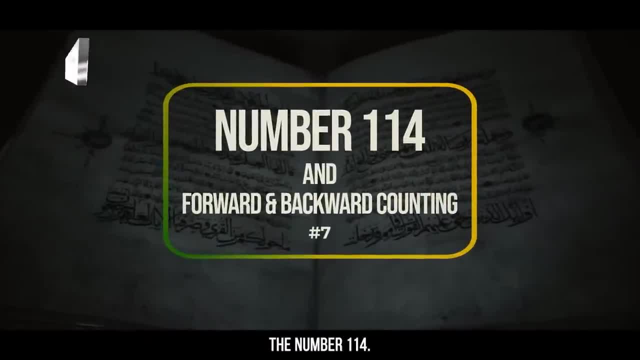 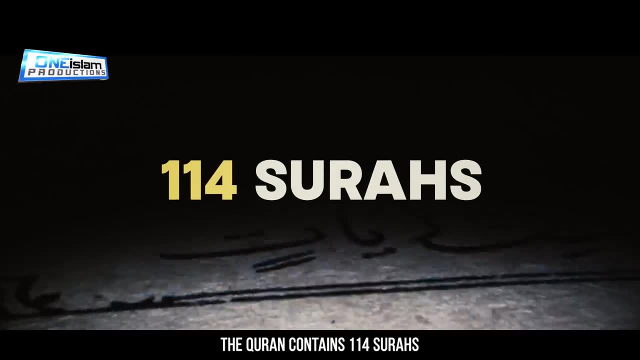 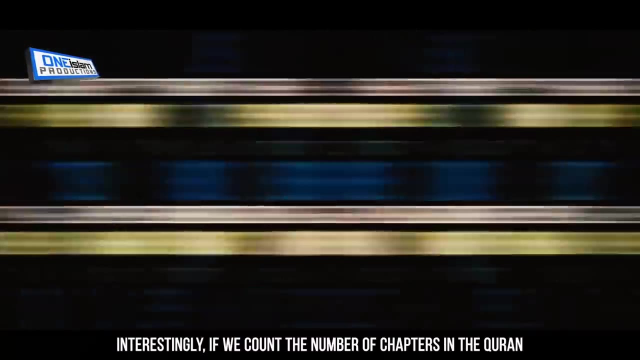 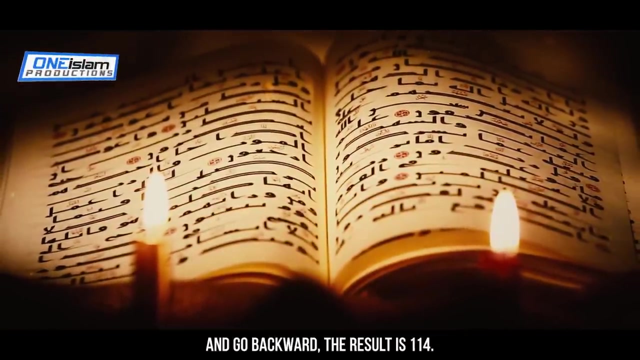 seven, the number 114 and the forward and backward counting. the quran contains 114 surahs and this number has been the subject of various numerical studies. interestingly, if we count the number of chapters in the quran, starting from the last chapter, surah nas, and go backward, the result is 114.. this phenomenon is 214.. 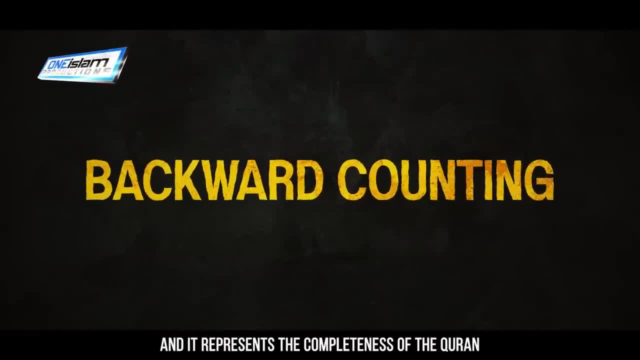 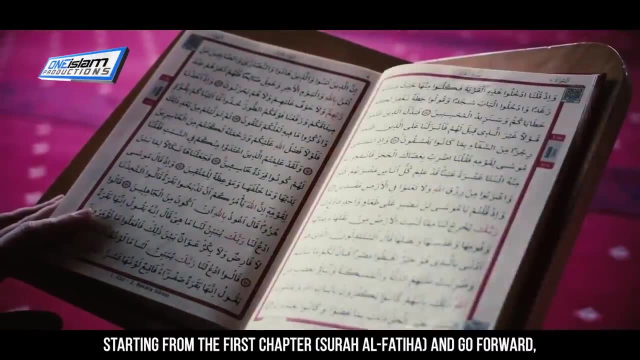 This phenomenon is called the backward counting, and it represents the completeness of the Qur'an. In addition, if we count the number of chapters, starting from the first chapter, Surah Al-Fatiha, and go forward, the result is also 114.. 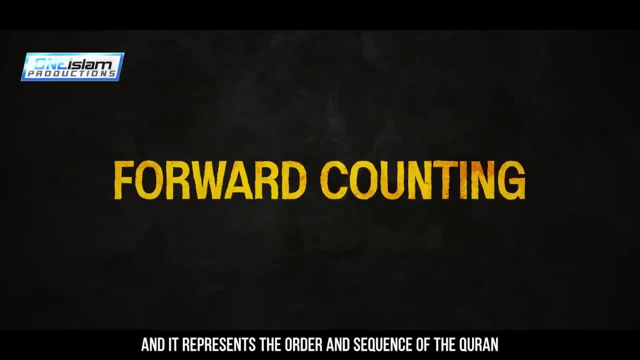 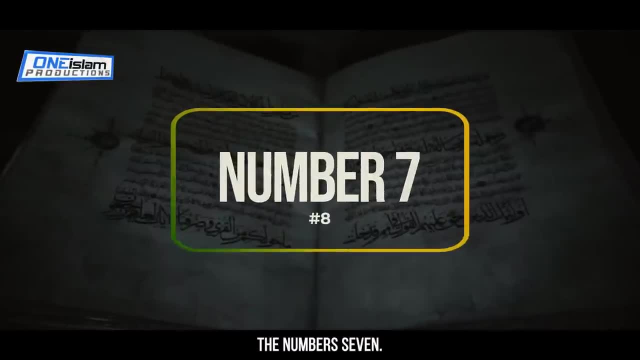 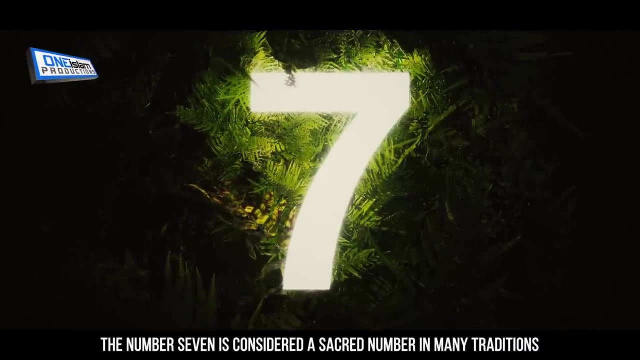 This phenomenon is called the forward counting and it represents the order and sequence of the Qur'an 8.. The number seven in the Qur'an. The number seven is considered a sacred number in many traditions and cultures. It is found in the Qur'an in many forms and contexts. 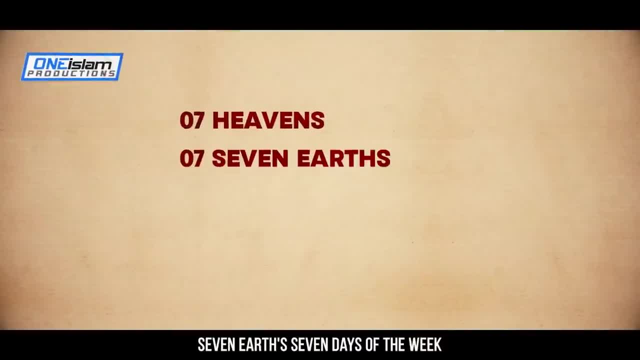 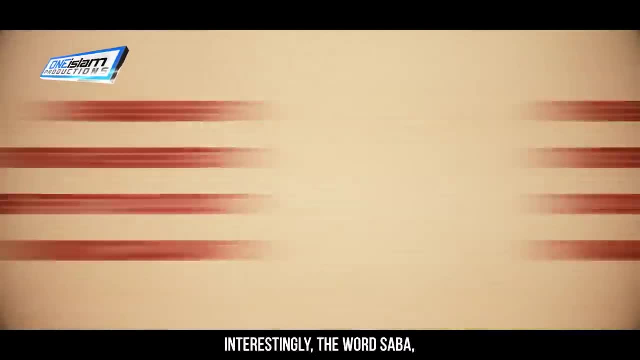 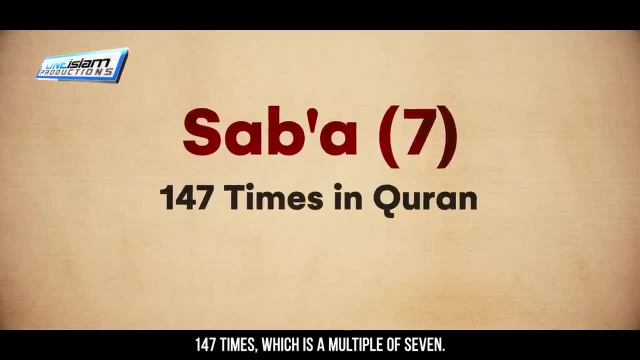 For example, there are seven heavens, seven earths, seven days of the week and seven major sins. Interestingly, the word سبع, which means seven, appears in the Qur'an one hundred and forty-seven times, which is a multiple of seven. 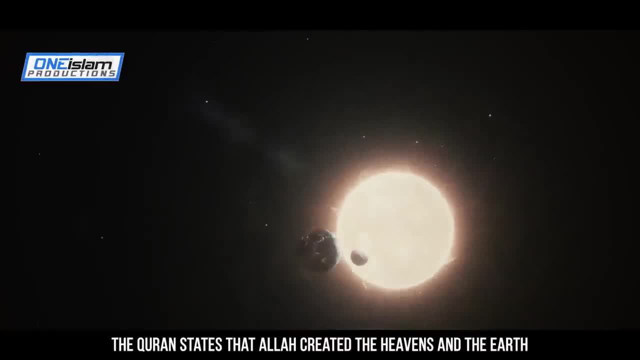 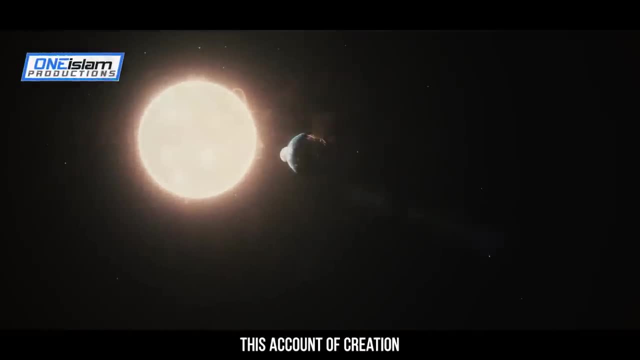 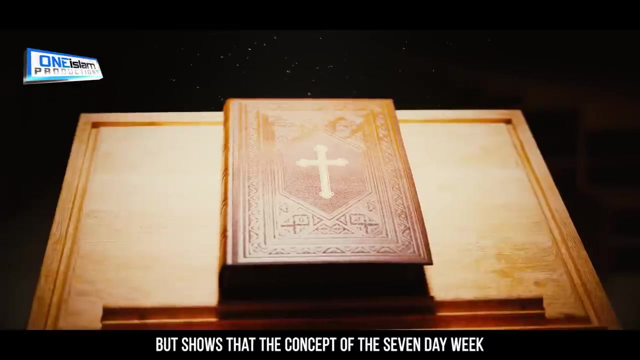 Furthermore, the Qur'an states that Allah created the heavens and the earth in six days and then established on the seventh day. This account of creation is similar to the Genesis account in the Bible, but shows that the concept of the seven-day week is older than Judaism or Christianity. 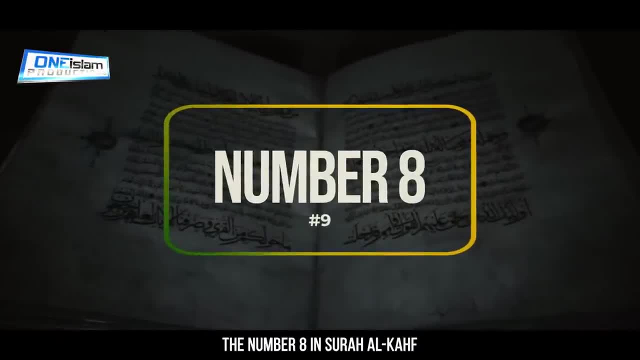 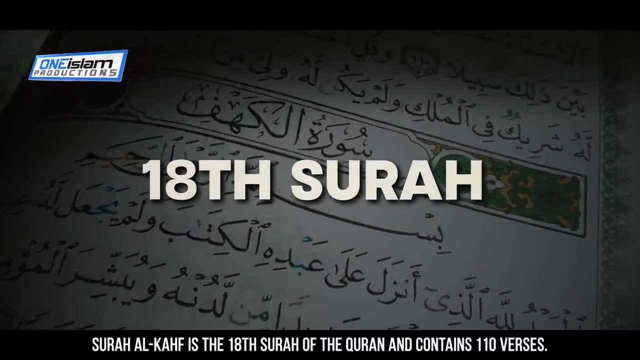 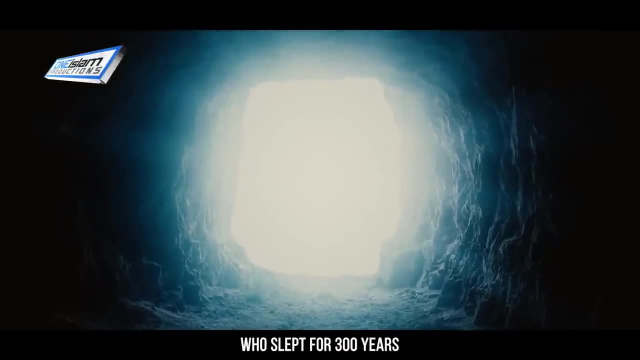 9. The number eight in Surah Al-Kahf. Surah Al-Kahf is the eighteenth surah of the Qur'an and contains 110 verses. This surah tells the story of the people of the cave who slept for three hundred years. 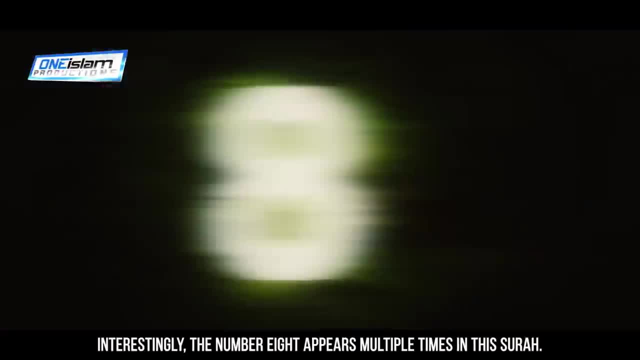 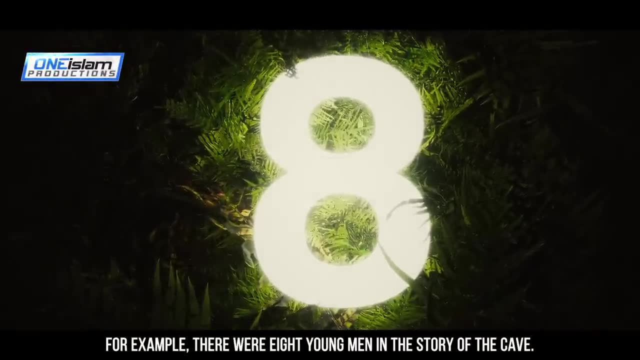 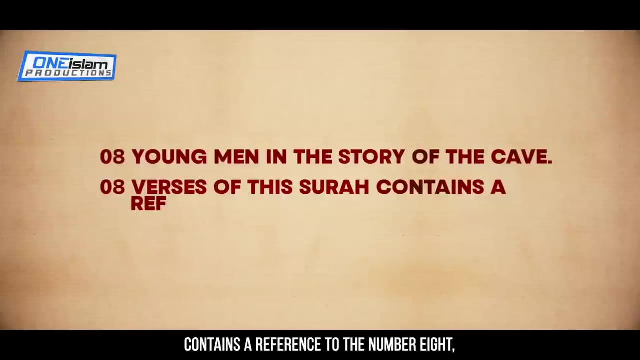 and other stories that teach important lessons. Interestingly, the number eight appears multiple times in this surah. For example, There were eight young men in the story of the cave. In addition, the eight verses of this surah contains a reference to the number eight. 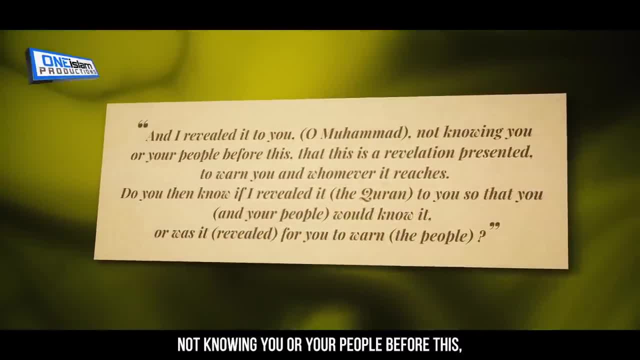 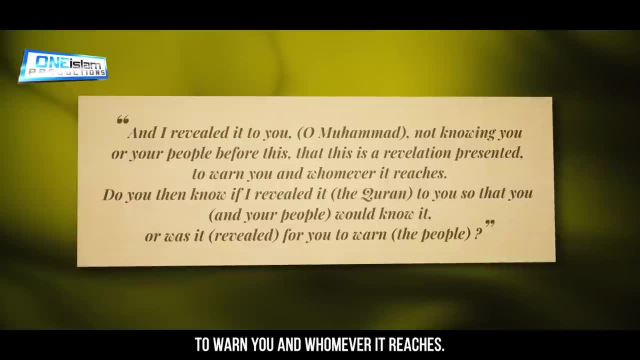 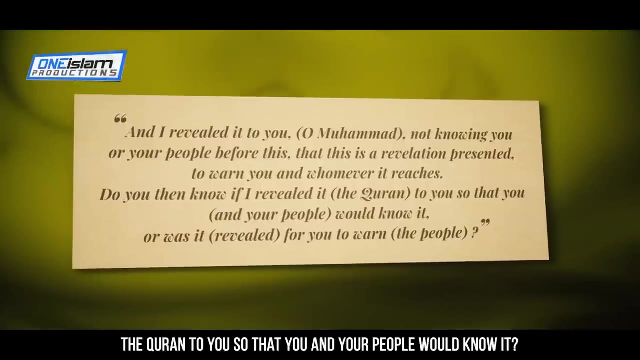 And I revealed it to you, O Muhammad, not knowing you or your people before this, that this is a revelation presented to warn you and whomever it reaches. Do you then know if I revealed it- the Qur'an- to you so that you and your people would? 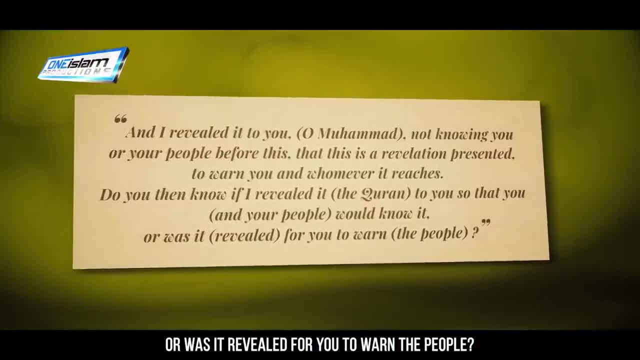 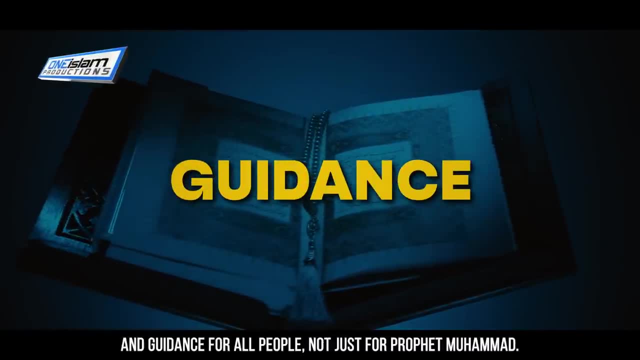 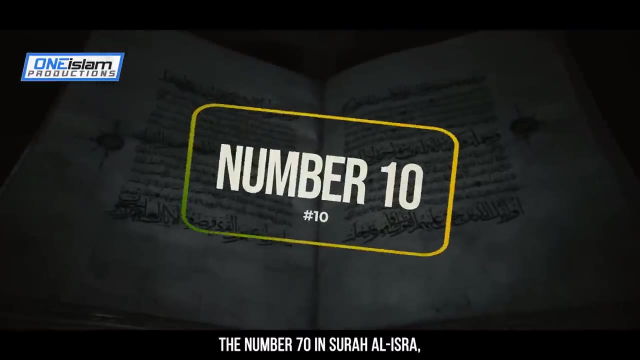 know it Or was it revealed for you? Did you know that the Qur'an is the first surah of the Qur'an? This verse teaches that the Qur'an was revealed as a warning and guidance for all people, not just for Prophet Muhammad and his followers. 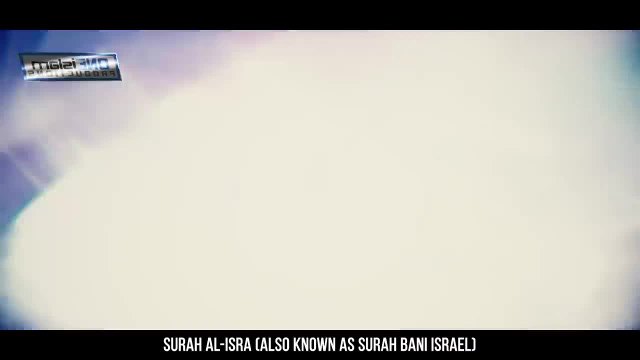 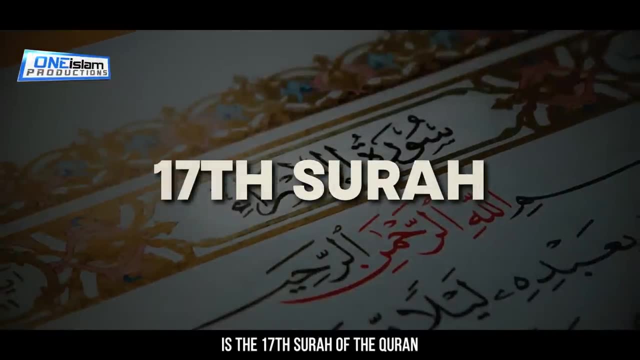 10. The number ten in Surah Al-Isra. Surah Al-Isra, also known as Surah Bani Israel, is the seventeenth surah of the Qur'an and contains 111 verses. The Qur'an is also known as Surah Bani Israel. 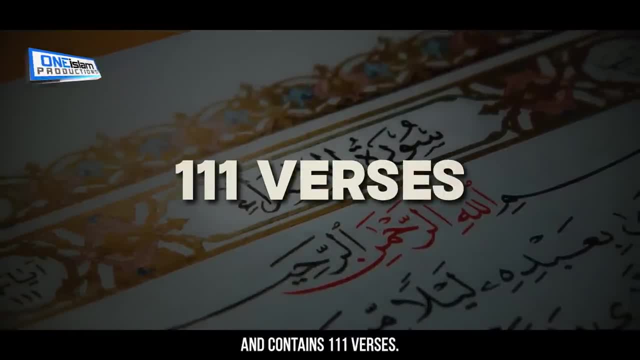 Surah Bani Israel is the seventh surah of the Qur'an. It contains 111 verses. Surah Bani Israel is the seventh surah of the Qur'an verses. This surah describes the Prophet Muhammad's miraculous journey to Jerusalem and other Prophet's. 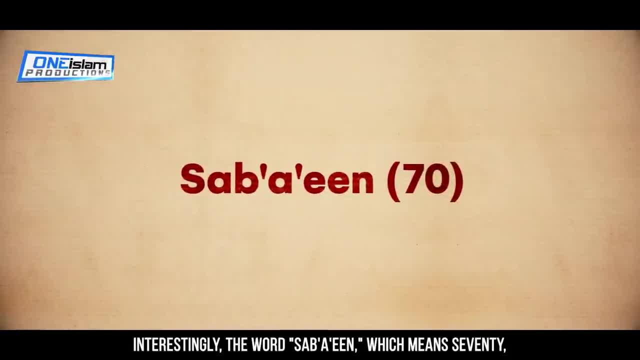 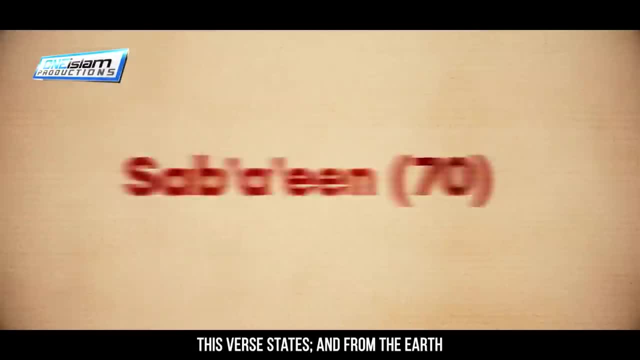 struggles. Interestingly, the word سَبْعِين, which means 70, appears in verse 5 of this surah. This verse states: And from the earth we have created you and into it we shall return you. 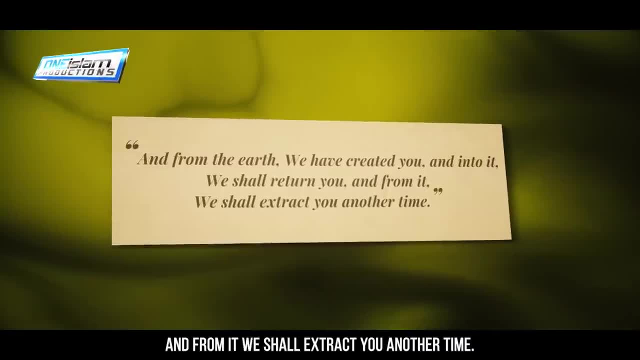 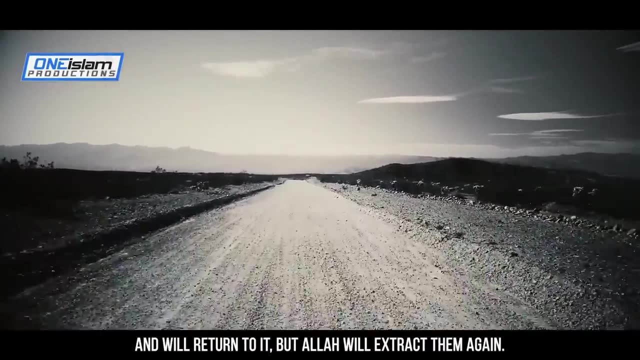 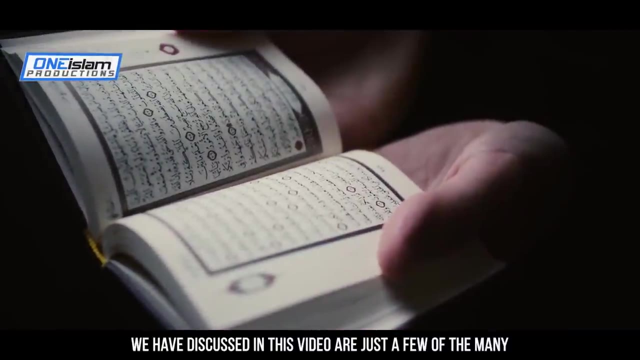 and from it we shall extract you another time. The essence of this verse is that human beings are made from the earth and will return to it, but Allah will extract them again on the Day of Judgment. The examples we have discussed in this video are just a few of the many that have been 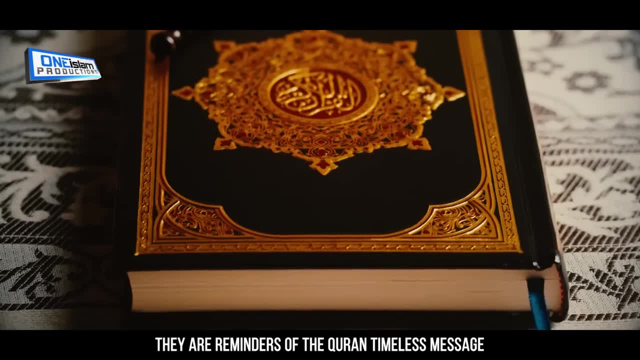 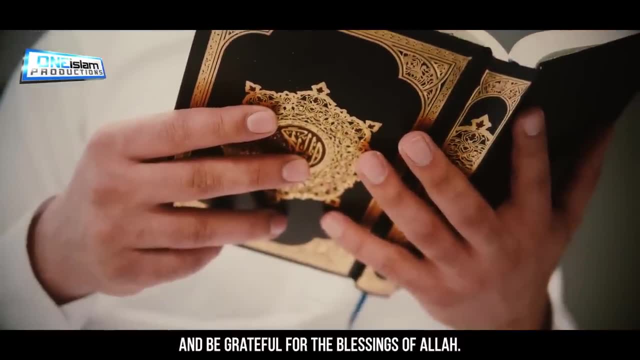 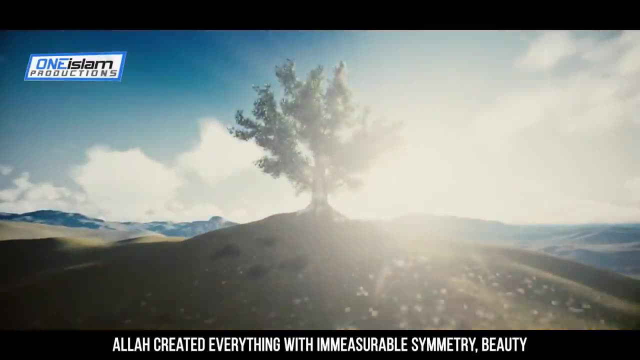 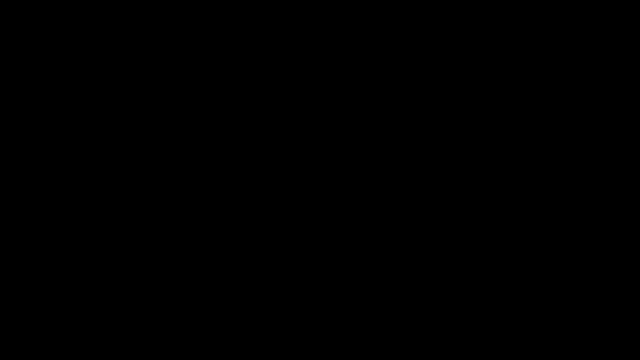 discovered by scholars over the centuries. They are reminders of the Quran's timeless message that invites us to reflect, Ponder and be grateful for the blessings of Allah. Allah created everything with immeasurable symmetry, beauty and perfection. Let the power of media improve your connection to your deen and make a positive impact on your life. 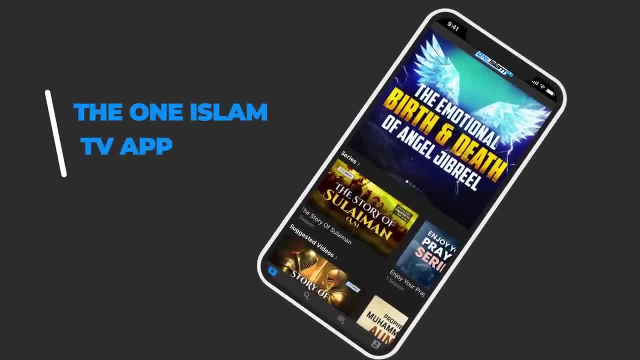 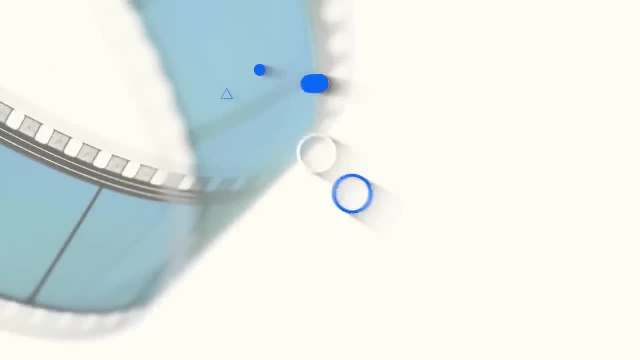 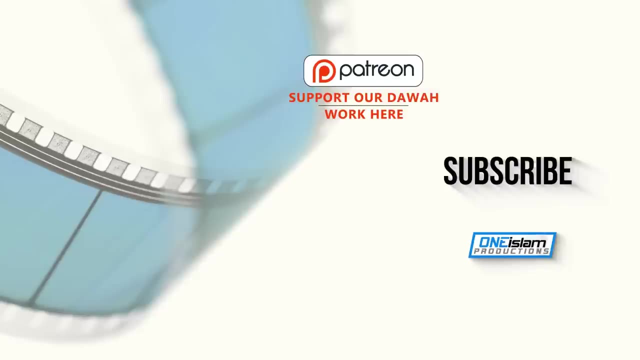 Download the OneIslam TV app today and embark on a transformative journey of knowledge, inspiration and spiritual growth. For more information, visit our website at wwwoshocom.